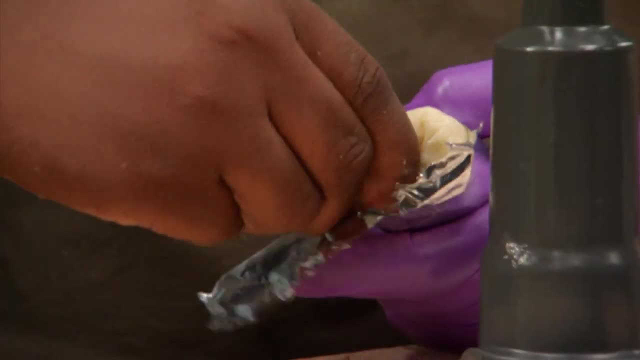 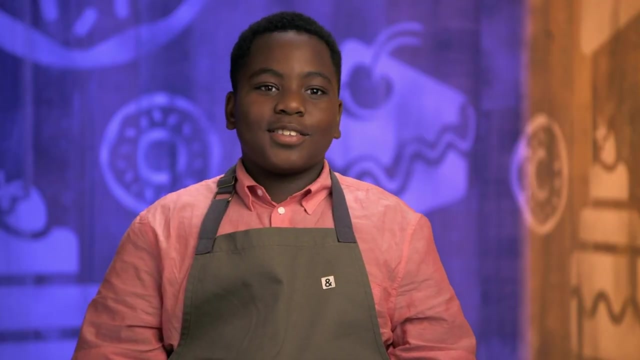 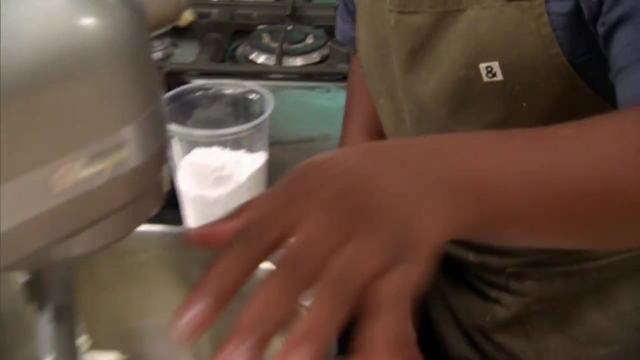 Oh, and don't forget the marzipan bakers. I've never used marzipan. That is good. I think I like this twist Secretly. I keep on eating. it Tastes like almond extract. It looks close to butter. 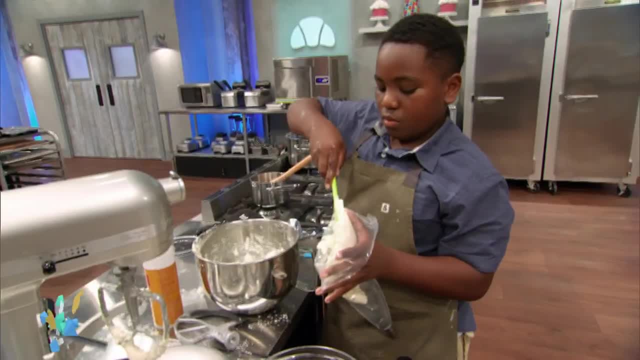 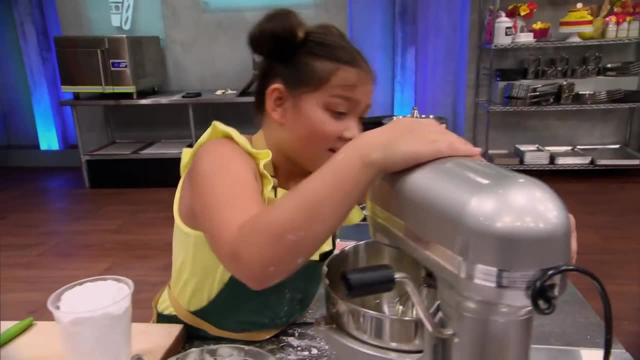 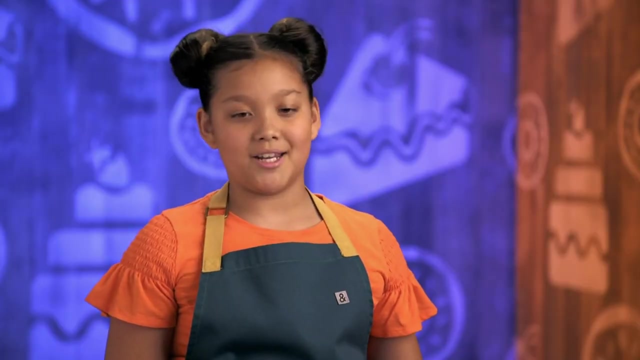 so I'm just going to make a marzipan buttercream. Yay, Who knows what to do with their marzipan? Not me, Not me. Duff and Valerie throw at us some weird almond dough that tastes really bad. My cupcakes are still in the oven. 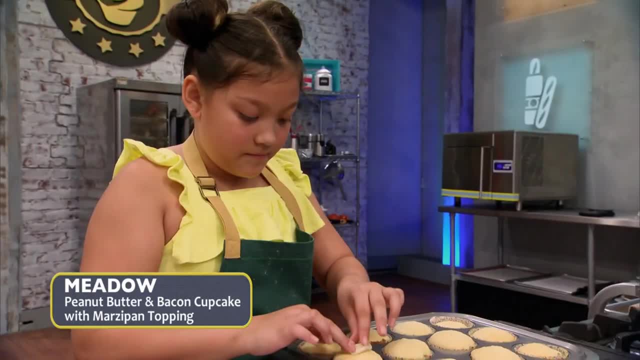 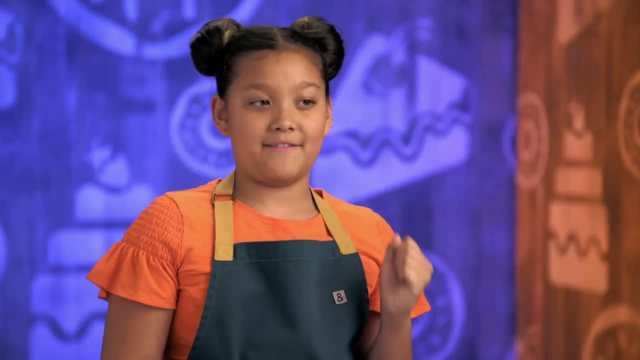 so I take them out and I just throw little sheets of it on top- They should get some in every bite if they take a big bite of it- And then I pipe on my peanut butter bacon frosting. I think that looks perfect. Can I just say these are the cutest cupcakes. 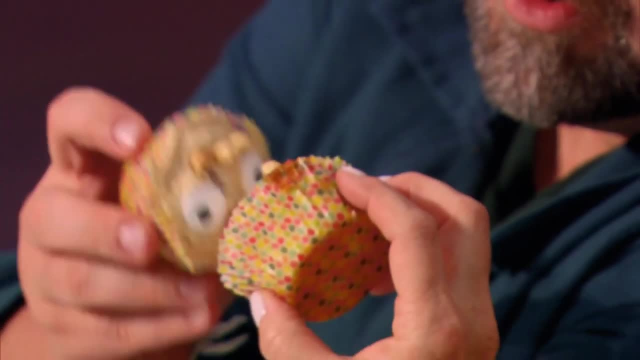 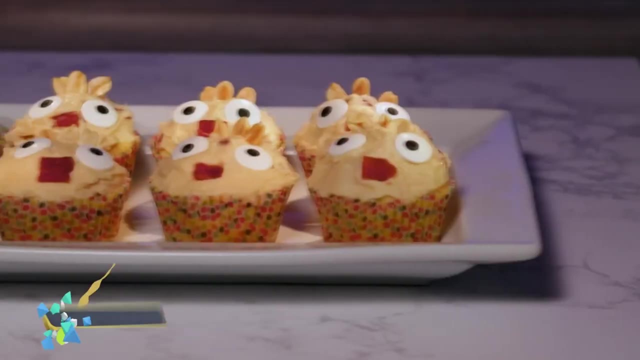 I've seen in a very, very long time. Caw, Caw, Caw. It's so cute, Meadow. what was your extra ingredient? A peanut. So I made a vanilla cupcake with a peanut butter bacon buttercream frosting. 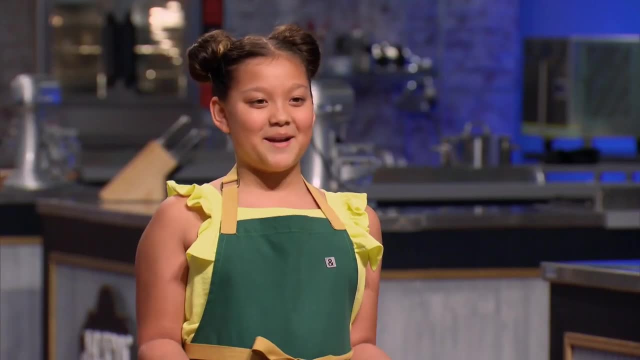 And the marzipan is on top of the cupcake. Yes, I made my cupcakes and then I took them out a couple minutes before they were done. I put a layer on top and then it kind of molded to the cupcake. 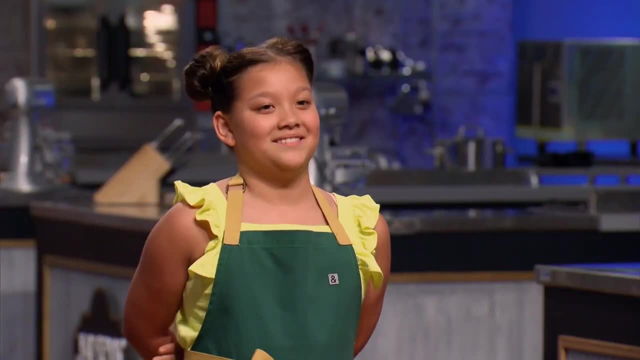 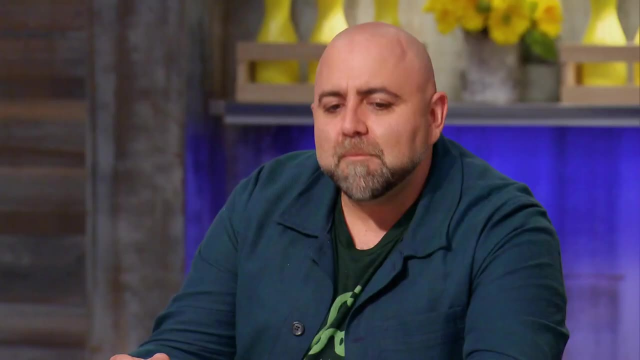 I 100% taste peanuts. I absolutely love peanuts. I absolutely get bacon and I actually get a very enjoyable amount of marzipan. You know the bacon, it could be a little crispier, I think, for this cupcake. 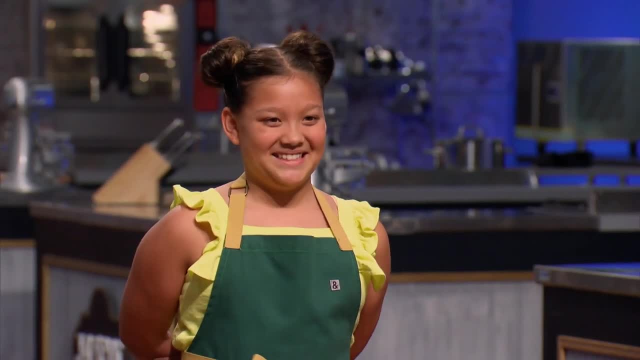 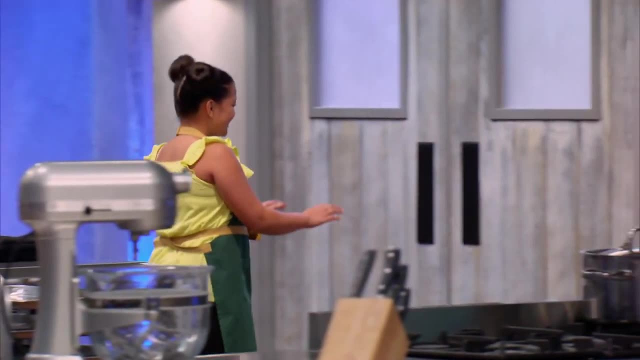 Maybe render it a little bit longer. Go you, I'm impressed. Thank you, Meadow. Thank you very much, Meadow. Cute hair, by the way. Thank you, I'm gonna do my hair like that. It's funny because I don't have any see. 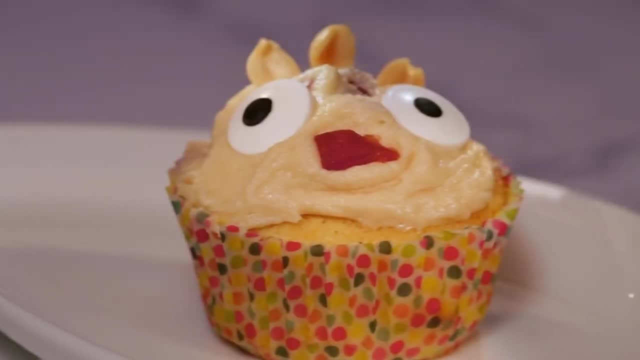 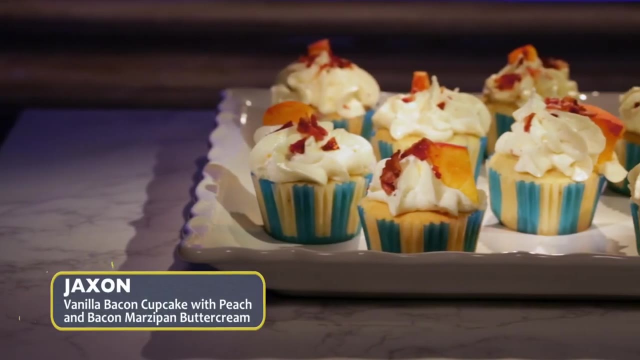 That was really enjoyable to eat. Mm-hmm Huh. Do you have a favorite ingredient in your cupcake, Texan? My extra ingredient was peaches, so I did a vanilla cupcake with bacon and a peach puree. 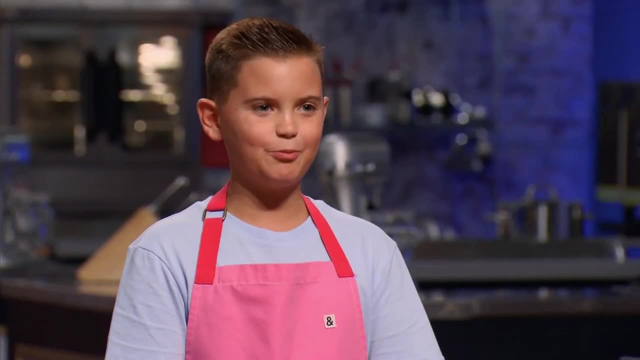 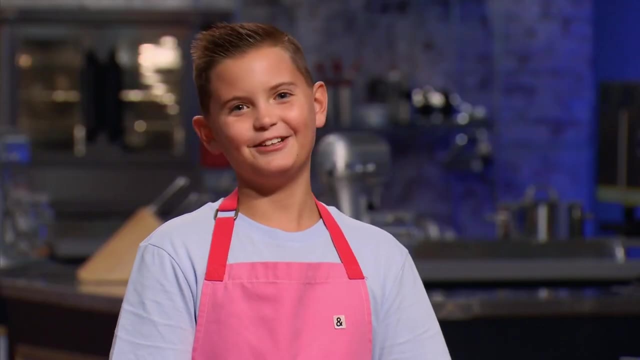 and then I did a marzipan and bacon buttercream. I've never tried a peach until probably today. Where do you live? In Mansfield, Texas. There's got to be peaches there. There is. I actually don't really eat fruit. 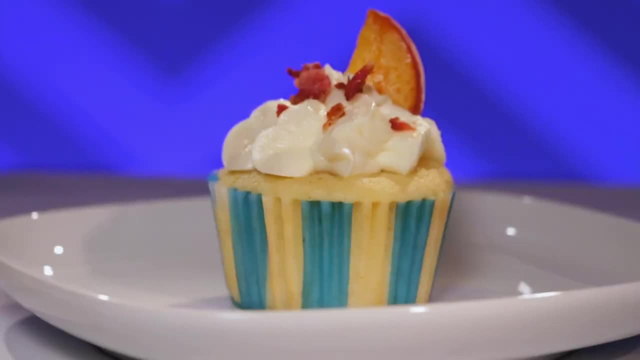 I'm a vegetable person. Well, I think your decorating is beautiful. Thank you. I love that you sprinkled it with bacon. You're telling me all the flavors that are in your cupcake, but I don't like it. It's coated by your decorations. 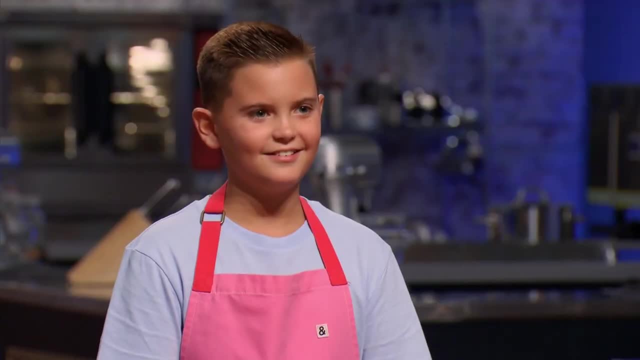 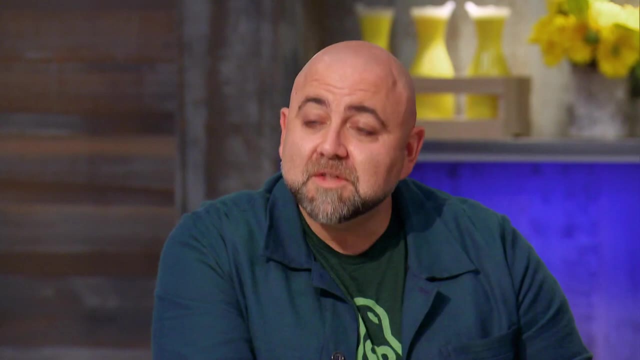 I do love the moistness of this cupcake, The peach puree. it gives the cupcake so much tenderness and moisture. It's really luscious in that way. Thank you, The peach flavor is great. You know, peaches are really difficult to get a flavor out of. 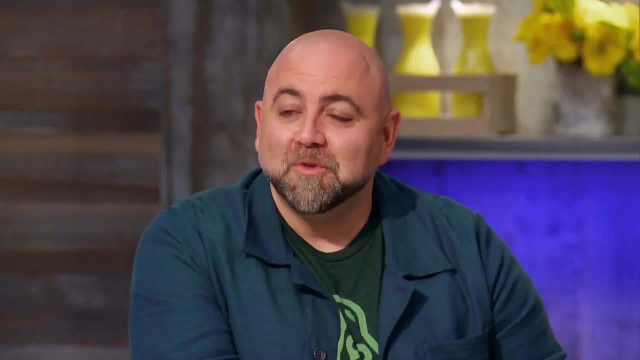 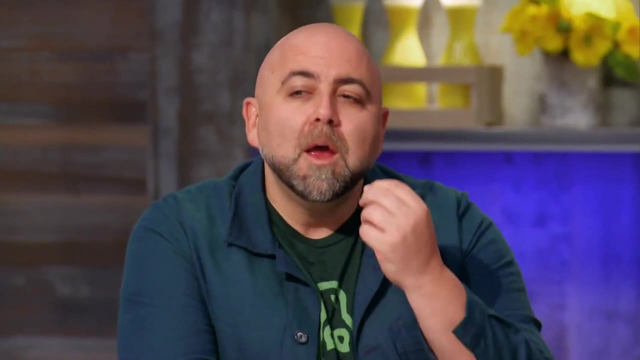 especially if you're somebody who's never had a peach before, or fruit for that matter. But it's really hard to taste the marzipan in there. I can feel the little chunks of it, but I really can't taste it OK. 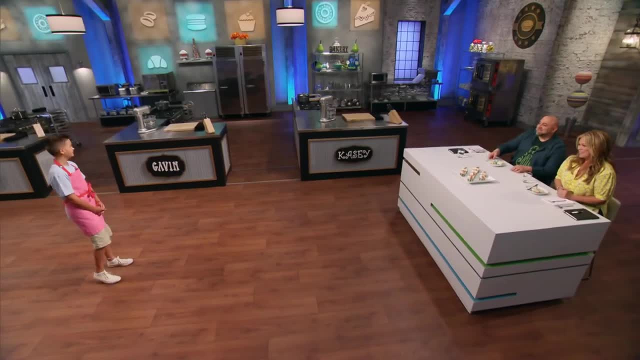 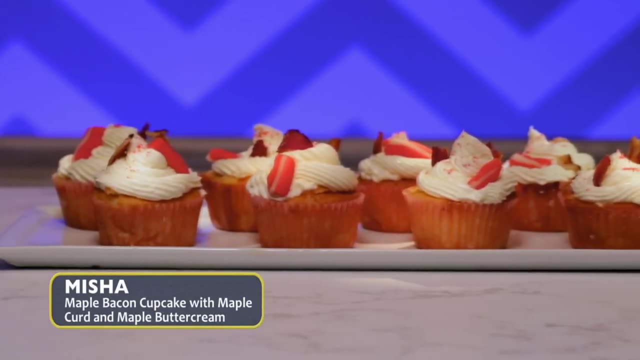 And also the cupcake and need a longer time in the oven. Thank you, Thanks, buddy. Thank you, Hey, Misha. My extra ingredient was maple, so I made a maple cupcake with bacon bits in it and a maple infusion curd. 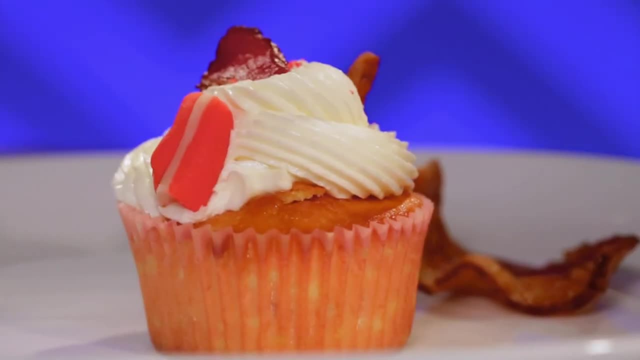 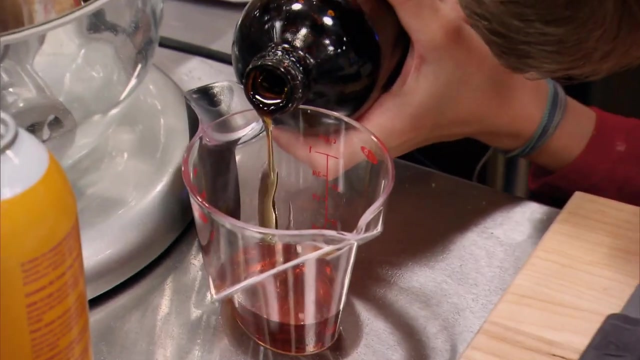 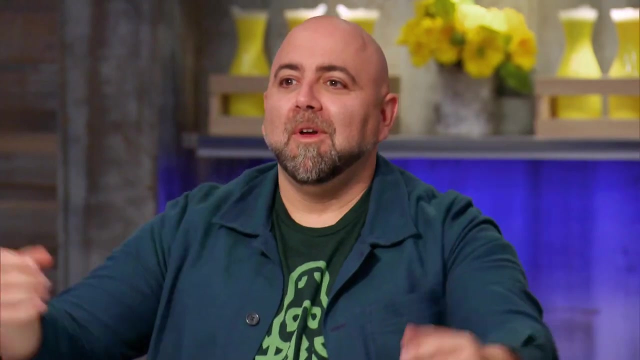 and I added maple to the buttercream as well as the marzipan for decoration. How'd you make a maple curd? I just used a normal lemon curd recipe and substituted the lemon juice for maple syrup. Ah, I'm excited about that. 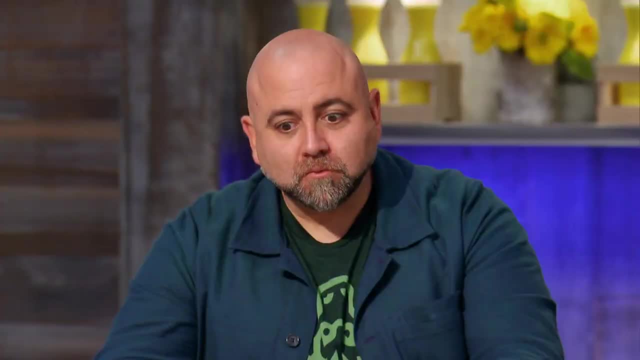 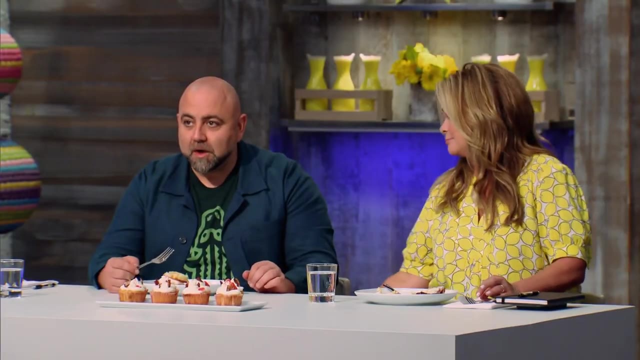 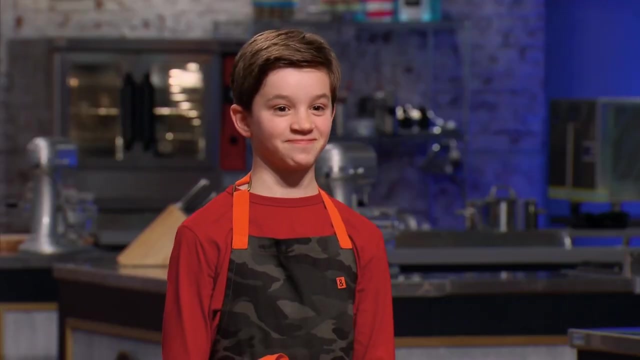 Mm-hmm, I say we go for it. This tastes like perfect pancake breakfast. Yes, You used real maple syrup in here. Yeah, You got the perfect amount. Wow, I'm so in love with this cupcake, but I would have liked to have seen. 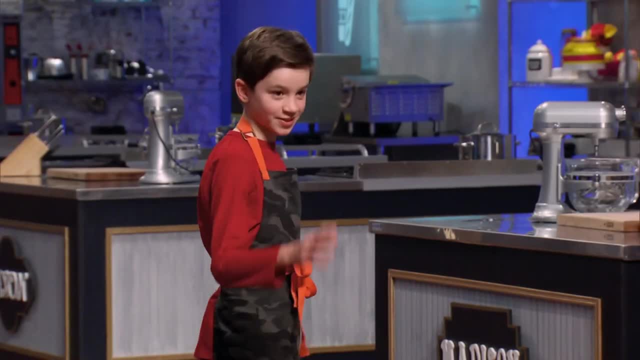 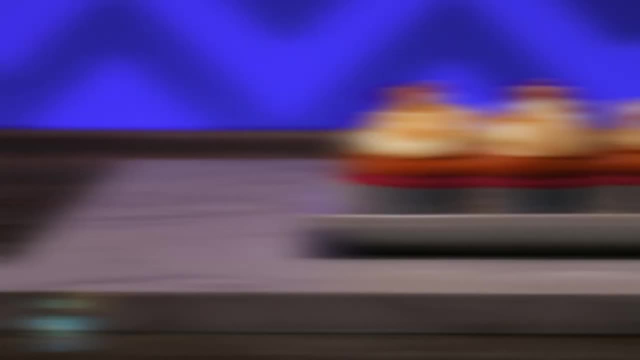 the marzipan incorporated a little bit more. Great job, ma'am. Thank you, Gavin. My ingredient was cinnamon, I used caramel and I made a bacon cupcake with a marzipan buttercream and a caramel drizzle on top. 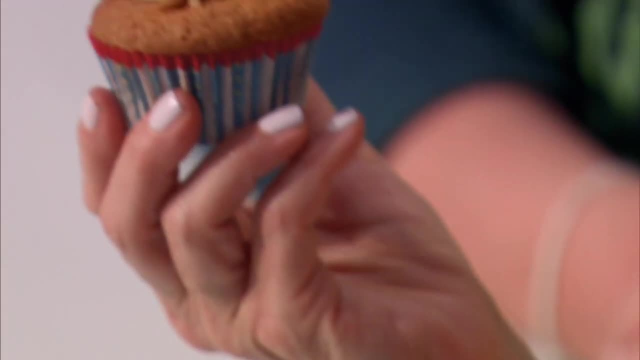 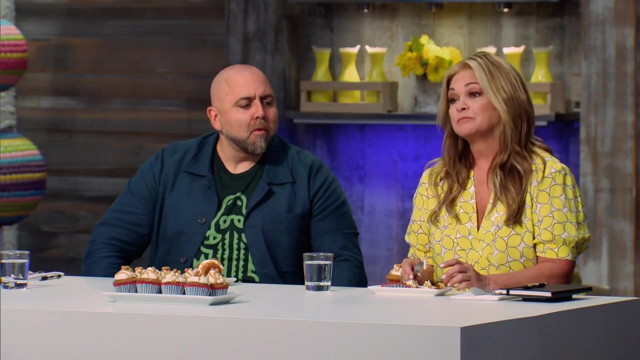 They're beautiful. They look like they could be in a window at a bakery. I'm super excited about trying this. Wow, That's a bacon cupcake. Uh-huh, Thank you. It's delicious. It's smoky and salty. 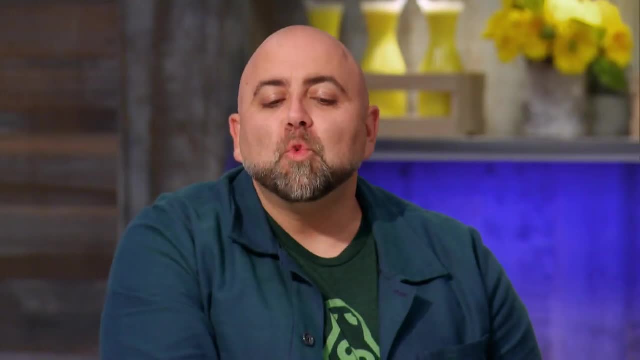 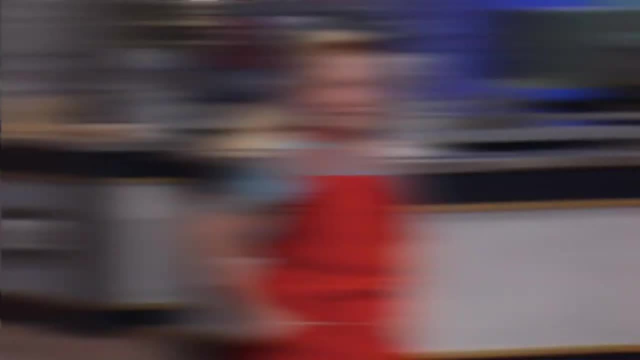 but yet I'm not getting a real strong marzipan flavor, though, Okay, I'm not really getting the caramel, because I just don't think it's dark enough. Okay, Thank you, Casey. Hello, What was your assigned ingredient to mix with the bacon? 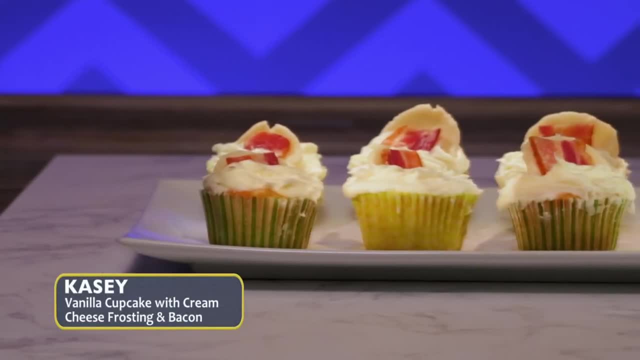 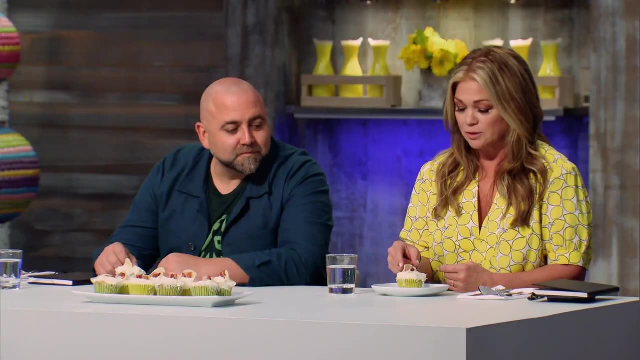 Cream cheese. So it's a vanilla cupcake with cream cheese frosting and I wrapped the bacon in the marzipan so it kind of looks like a shell. Oh, you mean this little wafer? Yeah Yeah, It looks like my communion wafer. 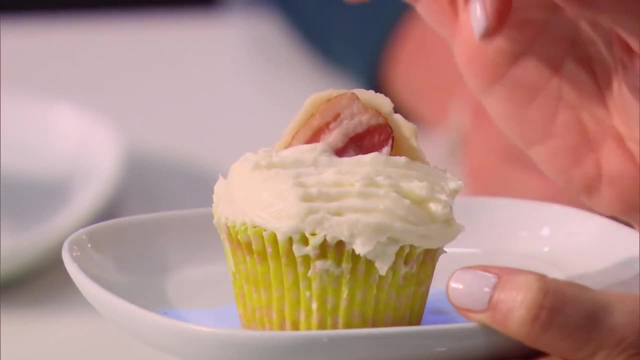 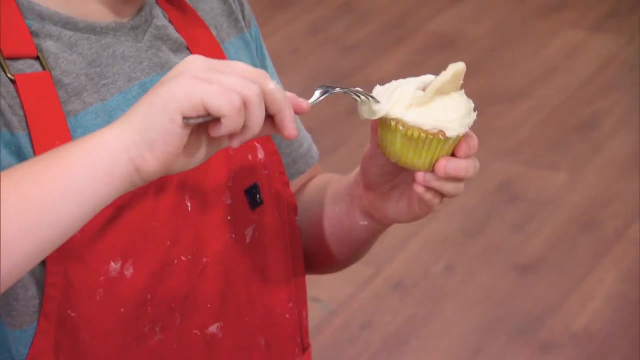 I don't understand why you started taking the fork and playing with the icing because it makes it look a little messy. The piping wasn't really working Like it was a little too soft for that, so I put the fork through it and I thought it would look like waves. 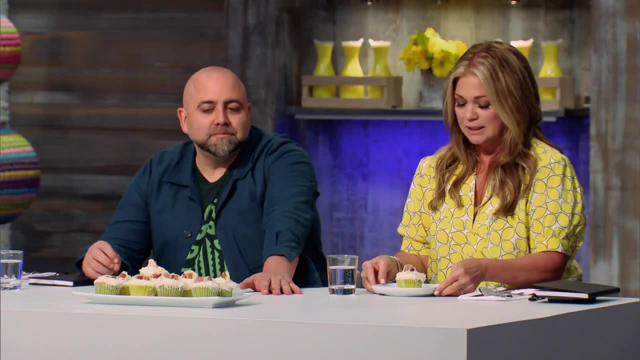 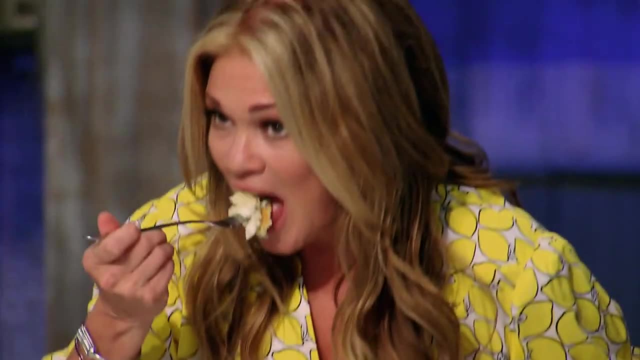 so it's kind of like an ocean theme. Oh okay, Wow, A little messy though, Yeah, But I think now we should try it. I think so too. It's a good cream cheese frosting, a good vanilla cupcake. 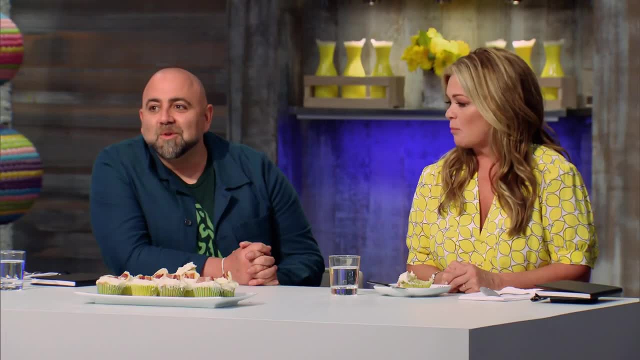 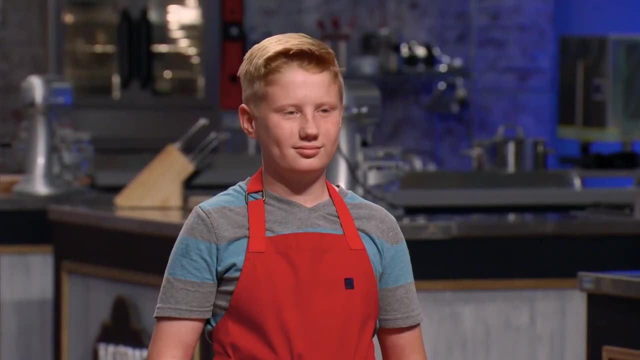 but I need you, to be honest, I want you to be a little more creative. Okay, You know what I mean. Like, think about ways to get the bacon and marzipan in here. That would be pretty cool, Mm-hmm. 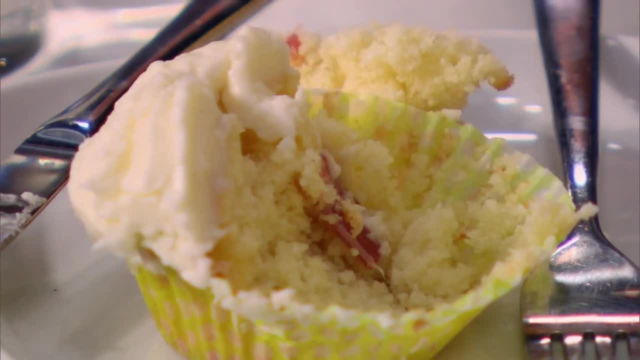 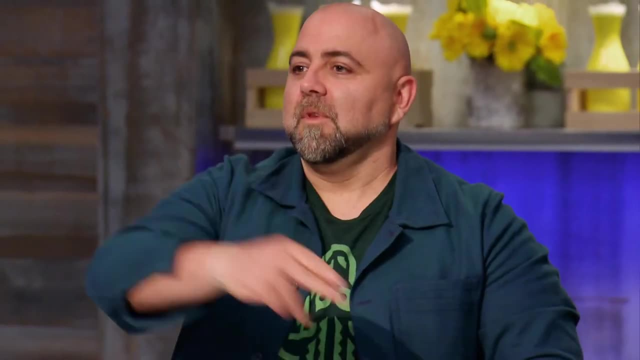 I wish that there was more bacon flavor in there, you know, incorporated through the cupcake. I do really love your cream cheese frosting, though. It's delicious. Thanks, Kasey, Thank you, Thank you. See ya, After judging, I'm not feeling very good. 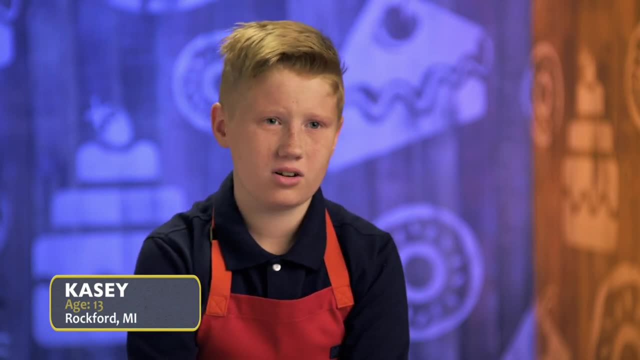 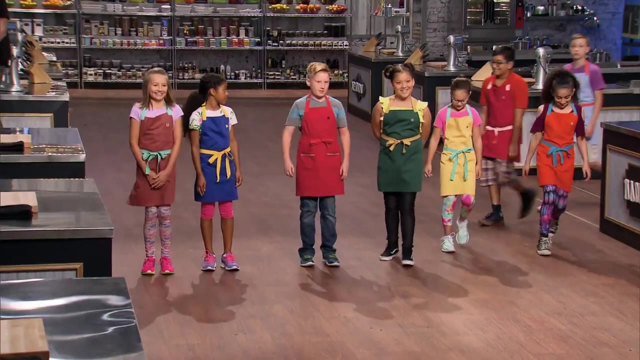 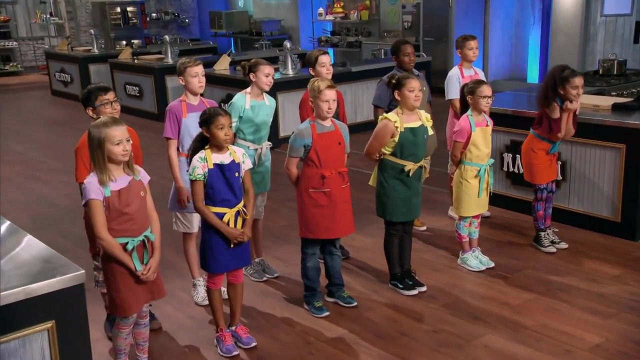 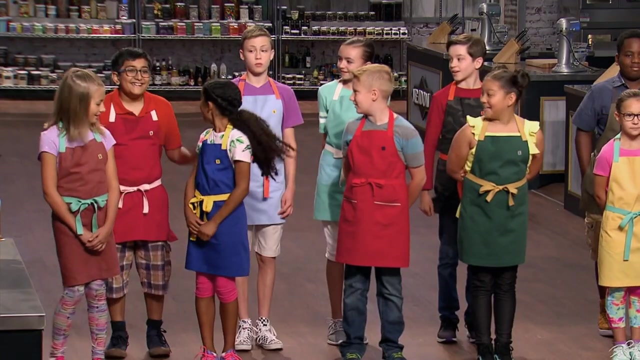 I made a couple mistakes and it's my first bake and I really hope I get to go to the next round. Bakers, your bacon cupcakes were awesome and three of you baked your way to the crispy crunchy top. Karthik, your cherry cupcake was beautiful. 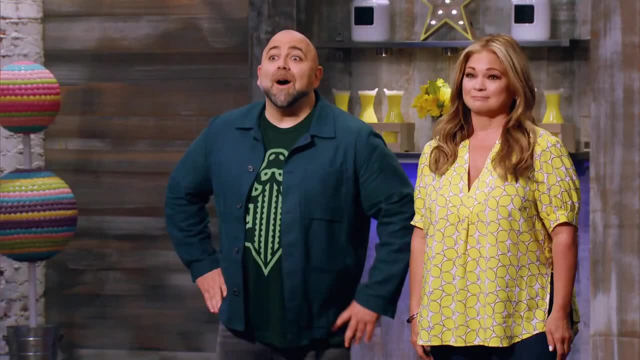 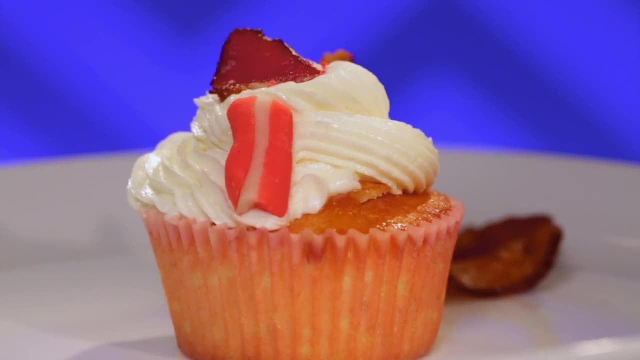 and your bacon buttercream made us both say, wow, Thanks, Misha. Yes, Come on, Misha, Your maple bacon cupcake tasted like a breakfast. It tasted like a breakfast cupcake in the best possible way, Thank you.